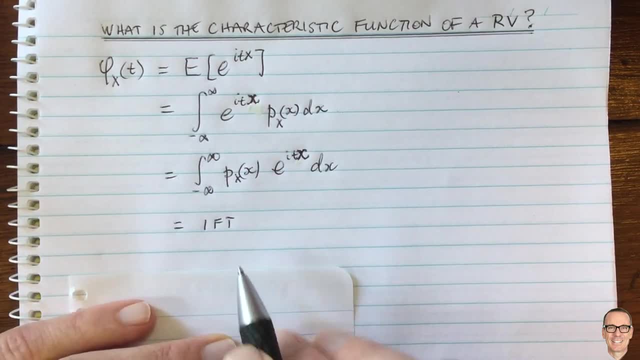 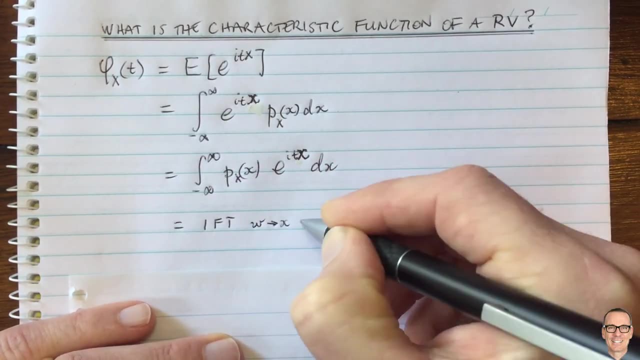 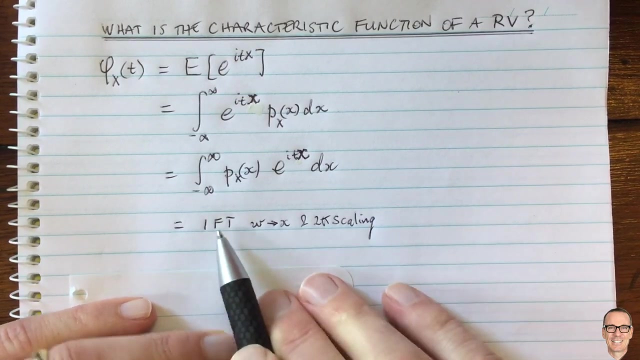 x and there's also a scaling of 2 pi. So this is the inverse Fourier transform. I'll just- I'll just indicate this with omega replaced by x, and and I'll put the 2 pi scaling here. So it's important that we just get that right for the to. 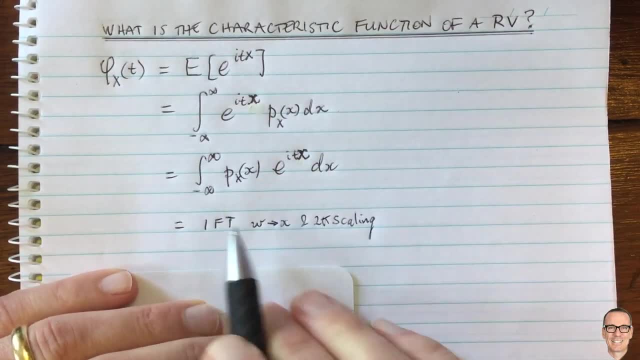 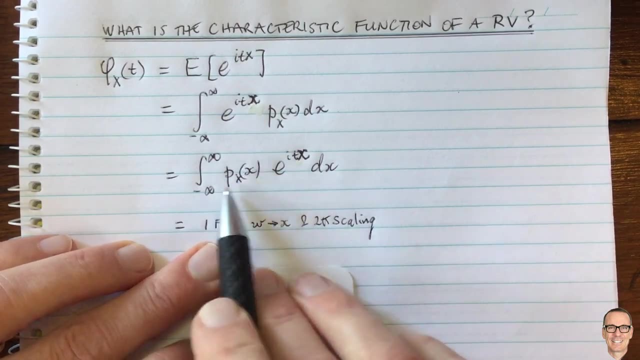 be exactly precise, But in fact it's just a scaling. so we this is a function of the form of inverse Fourier transform and of the pdf. So it's the inverse Fourier transform of the pdf, of the random variable. The characteristic function can be found or can go backwards and forwards between the pdf and the. 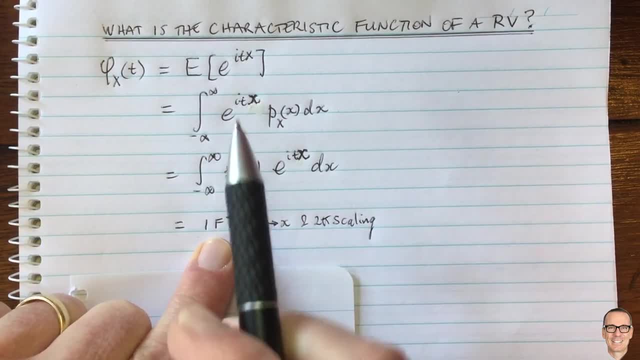 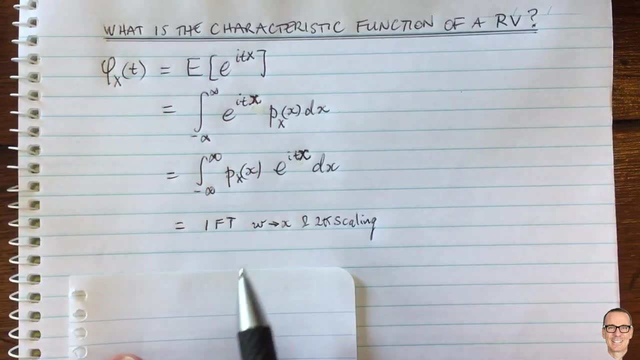 characteristic function using the Fourier transform. So if we had the characteristic function and we wanted to find what the probability density function is, then we could use the Fourier transform and, of course, go backwards and forwards. It's an invertible function, So that's a nice property. 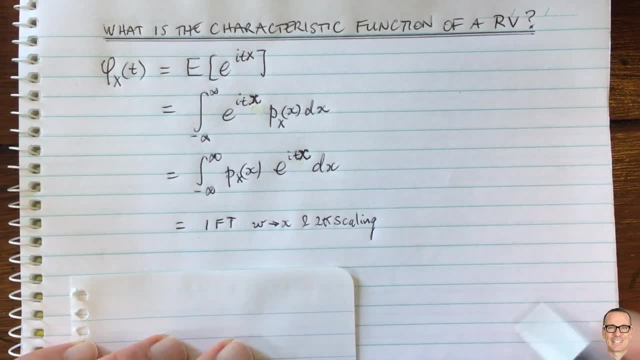 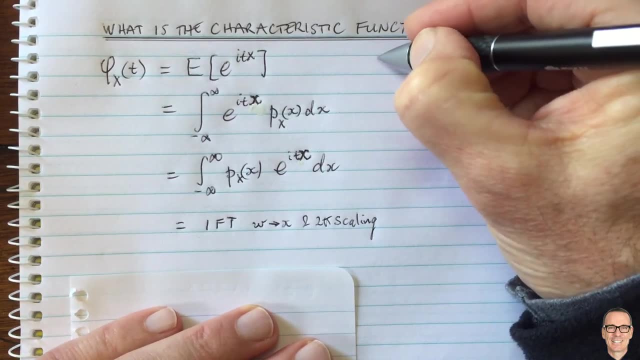 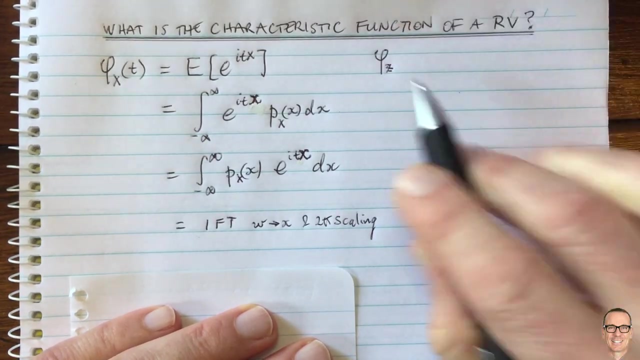 So why are we interested in this? Why do we use this? Well, we are often interested in adding random variables, So this is one of the uses of the characteristic function. So if we had another random variable, which was z, and we wanted to know about its pdf, then we could try to find its. 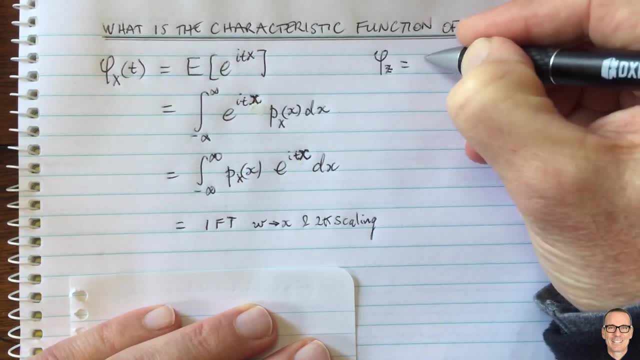 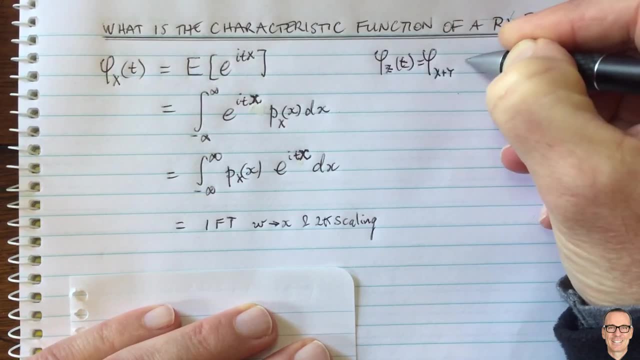 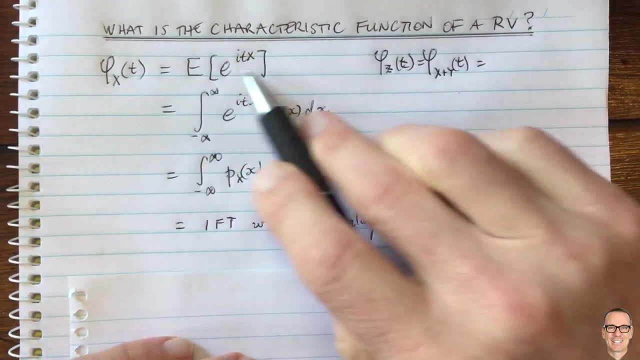 characteristic function. And how would we find that? Well, it's the characteristic function of x plus y, If we had z being x plus y. So let's think of a new random variable, z, which equals the addition of two other random variables. So in this case we can use this definition here and we can just simply write this in here: 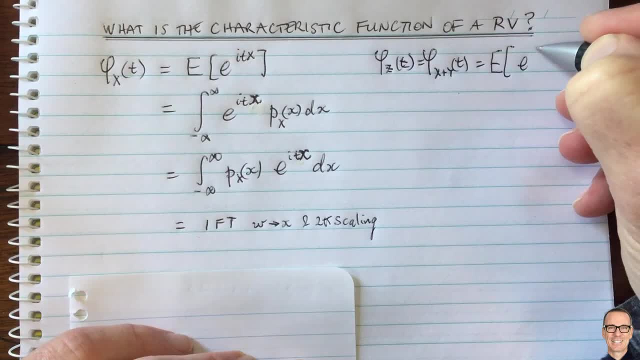 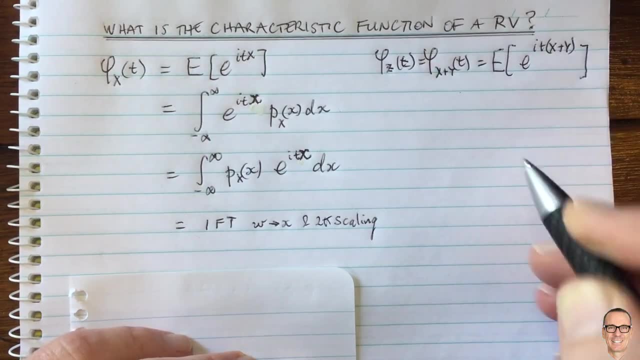 So in this case we can use this definition here and we can just simply write this in: here We've got the expectation of e to the power i, t, x plus y, Our new random variable, which is the addition of two others, And this happens very often in many random variable scenarios. Let's 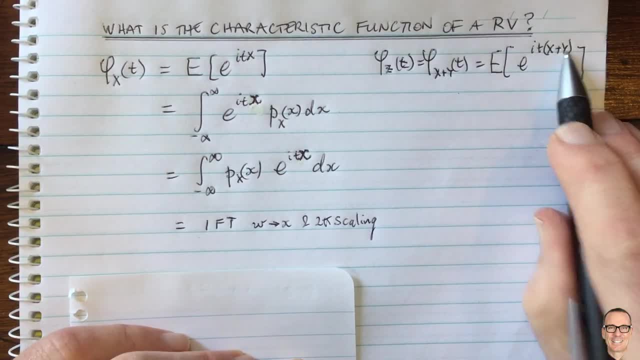 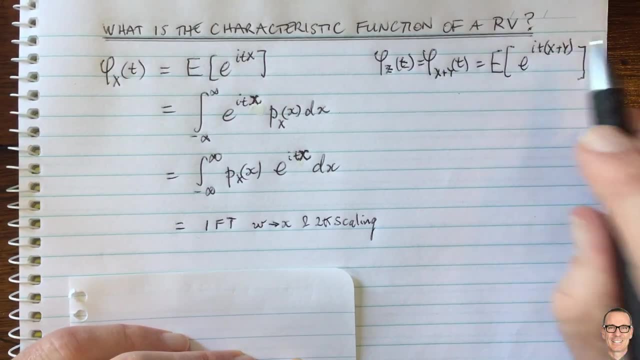 say digital communications, where you've got the data plus noise, or where there's two users, one user plus another user, So a symbol from one user plus a symbol from another user, And you're wanting to find out what the overall pdf is. And there's many other examples, of course. 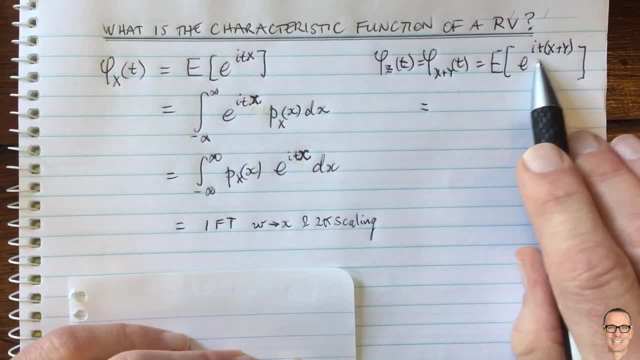 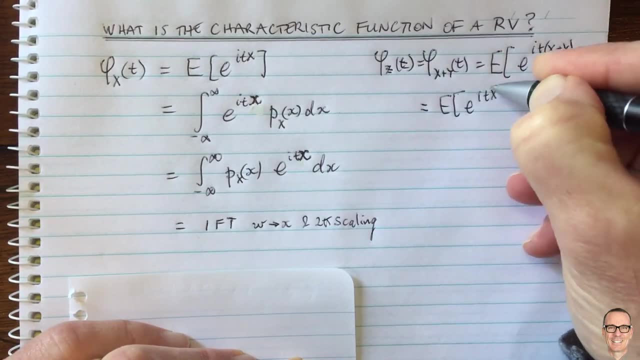 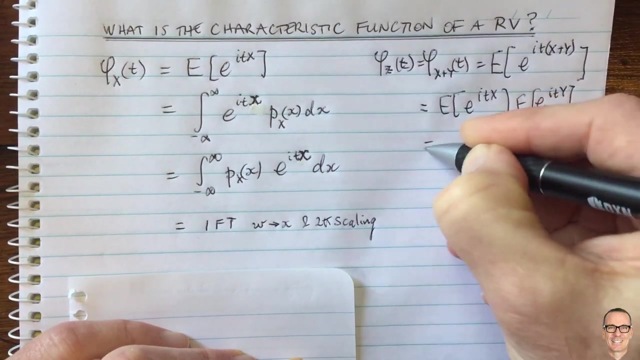 where you're adding random variables. So in this case here, if the random variables x and y are independent, then this equals the expected value of e to the i t x times the expected value of e to the i t y. So this equals, as you can see here, the characteristic function of x times the characteristic function. 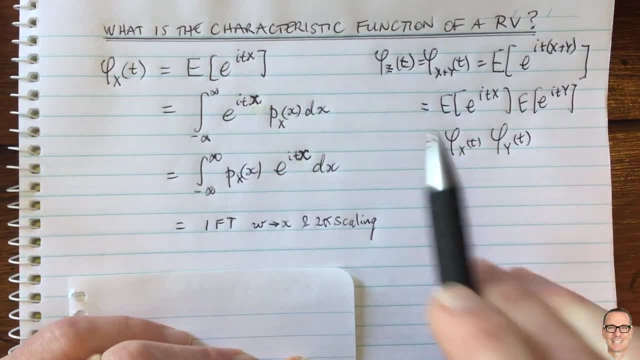 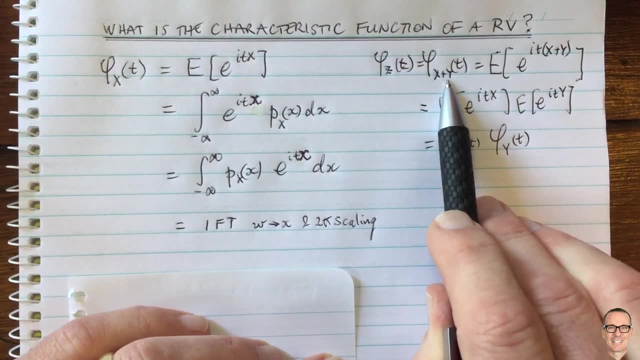 of y. So this is a very handy property because, as I say, if you're interested in the, what the properties of the i t x times the expected value of e to the i t y, So this is a very handy property. addition of two random variables is then you can work out its characteristic function very simply. 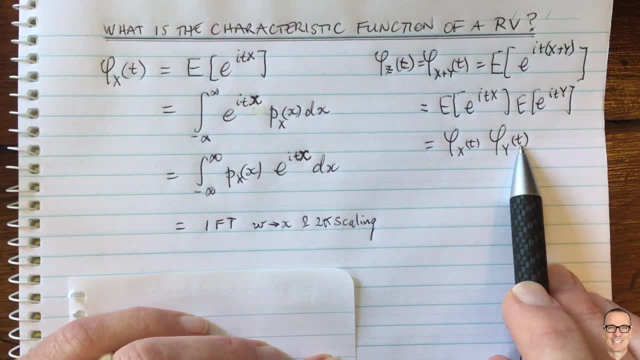 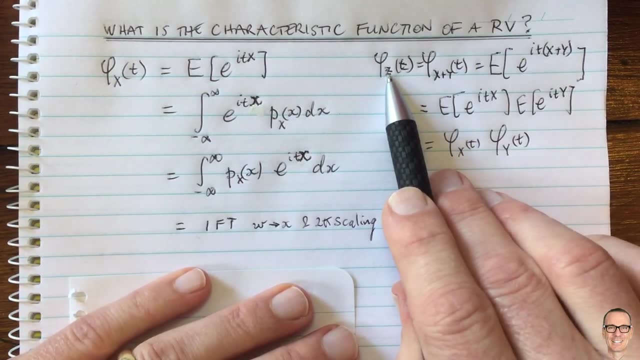 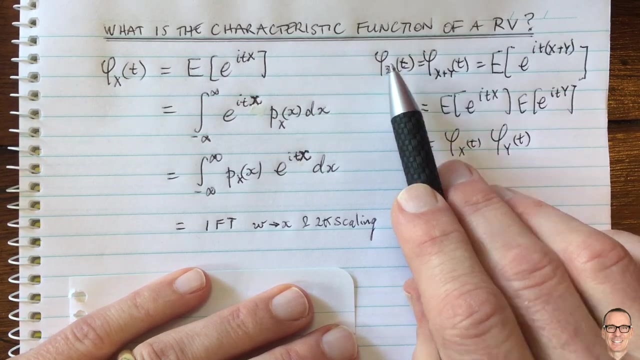 by multiplying the characteristic function of the two independent random variables. And then of course that means if you want the probability density function of z, then you can just simply perform this, find its characteristic function and then take the Fourier transform and you'll have the probability density function of z. If you weren't to do it with a characteristic function. 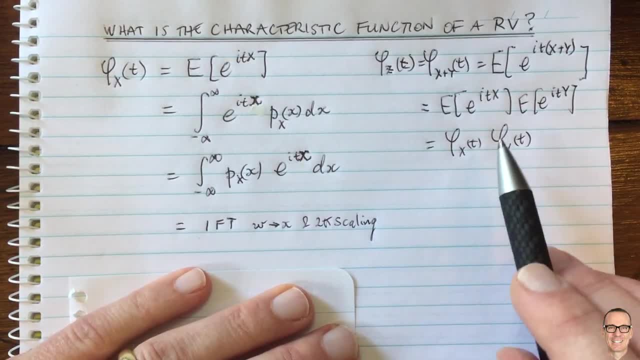 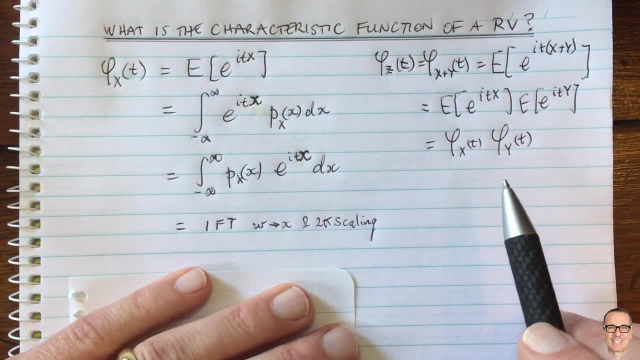 then you would have to take the characteristic function of z and you would have to take the convolution of the two probability density functions, The probability density function of x convolved with the probability density function of y. And we know that that's through the property. 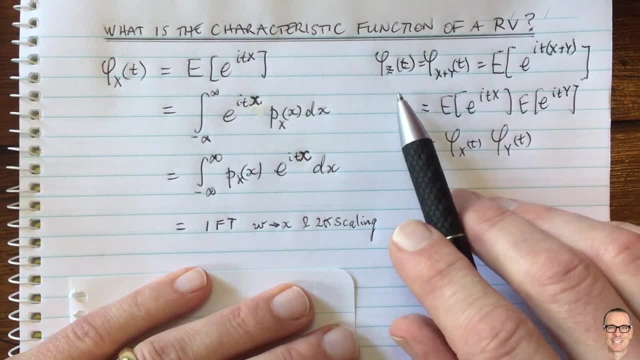 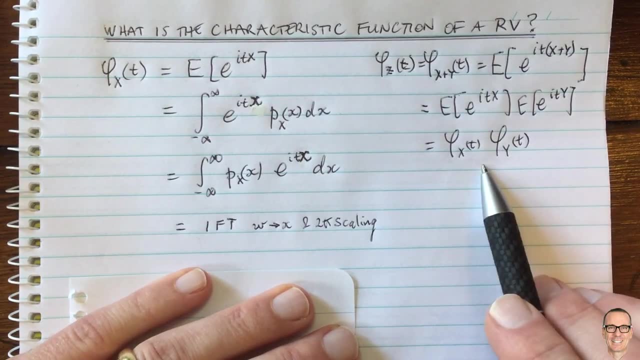 of one of the properties of the Fourier transform. If you have convolution in one domain, you have multiplication in the other, And here we've seen for the characteristic function it's multiplication. so if you were to do it without the characteristic function, you'd have to do the convolution. 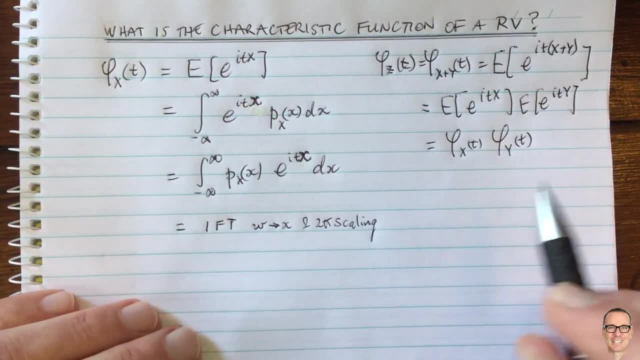 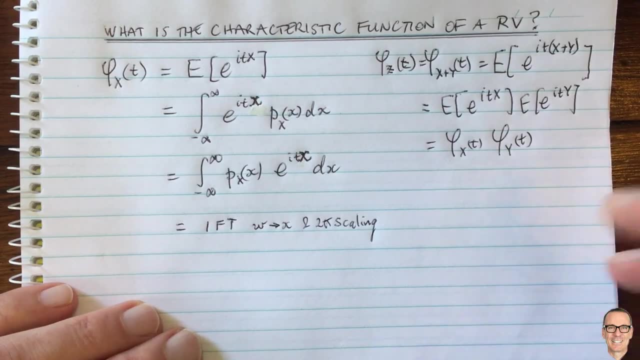 in the pdf domain and that would be more complicated often. So this is one of the uses of the characteristic function And I'll just point out one final thing here on maybe two other things. One thing is, if we put the parameter in there and we replace the t, with minus i of t, then this equals e of minus i squared. t x, which of course equals the i squared, equals minus one. So this of course equals e to the t squared. So this is a characteristic function, t x, and this equals the moment generating function. So we again another function, we're. 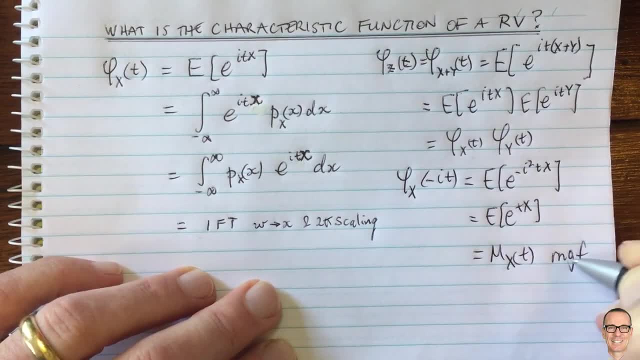 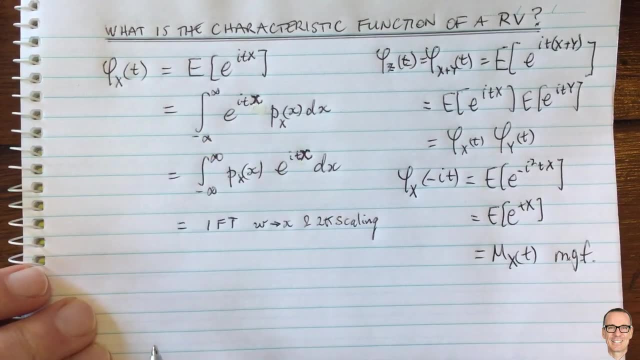 familiar with with random variables, the moment generating function, And again, there's a link below this video to that. And one final thing to note is that sometimes the characteristic function is defined in a slightly different way, So I'm going to write this out here with a prime above it. 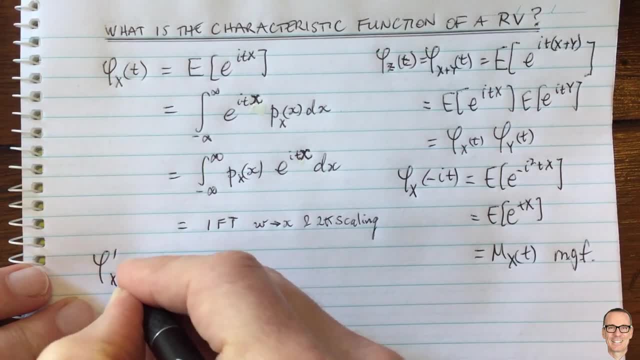 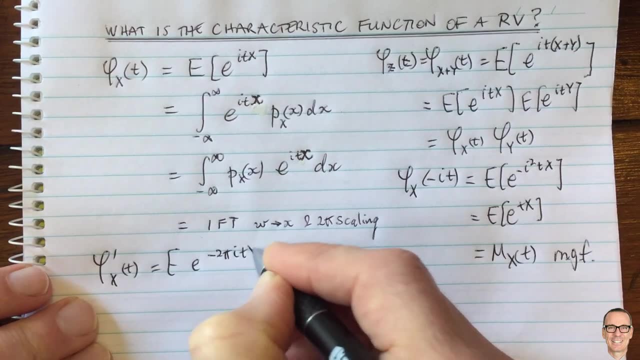 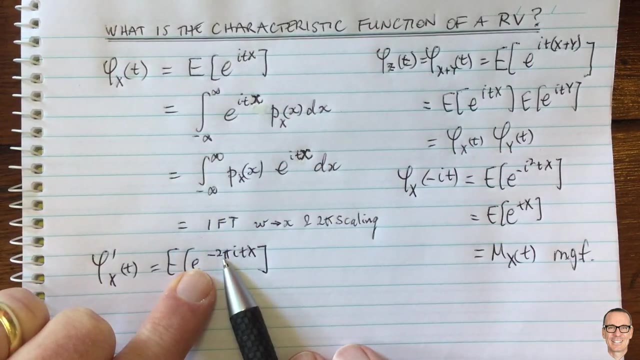 and it's sometimes defined to be this function here. So this is the expectation of e to the minus two pi, i, t of x. And with this definition, which is slightly different to this one, you can see there's a minus and there's the scaling of two pi And in 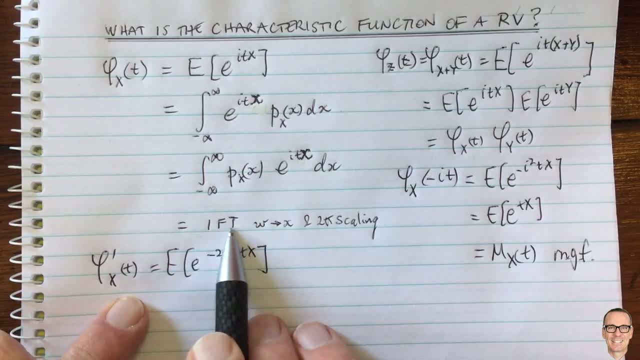 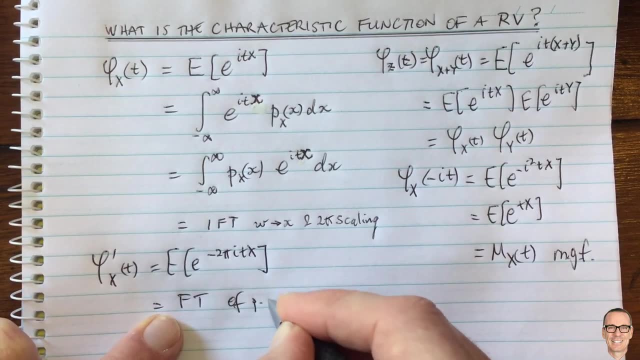 this case, then you're going to get, instead of the inverse Fourier transform, you're going to get the Fourier transform of the pdf in this case. So this is something, for I think you can put this into the formula yourself, into the expectation of e to the minus two pi, i, t of x, And with this definition, 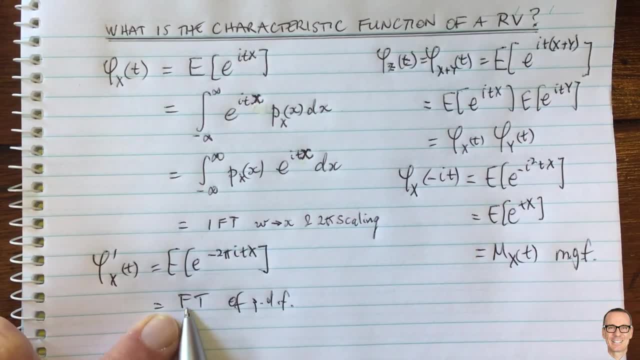 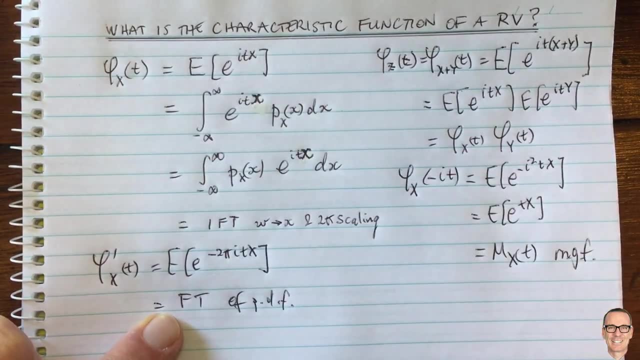 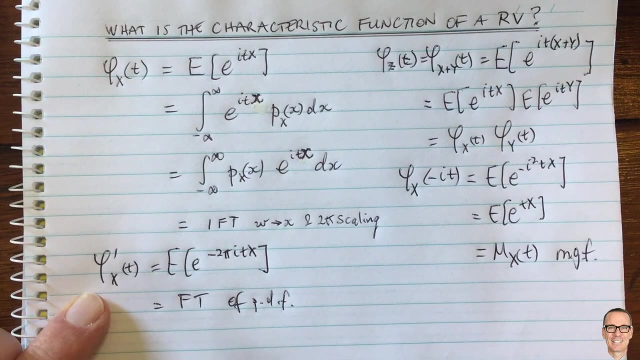 you get the Fourier transform instead of the inverse Fourier transform, And it's all because of putting this minus here, which we didn't have in this definition up here. So it's just important that you're aware of the fact that there is a different definition of the moment generating. 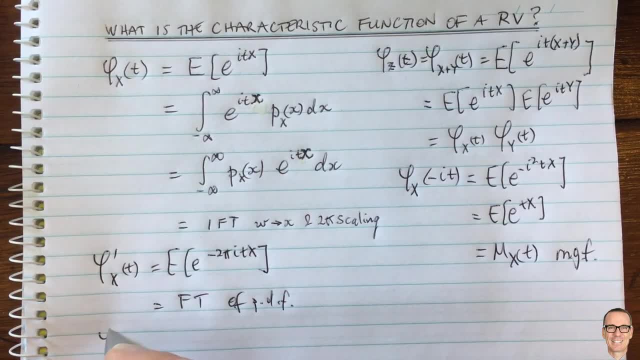 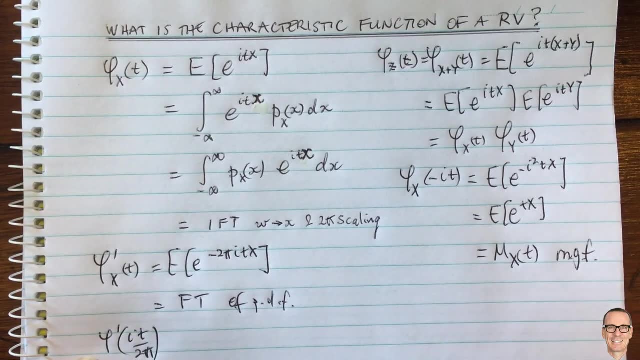 function. And again with this definition here. if we put in i t divided by two pi with this new definition, then we get the Fourier transform. And again with this definition here. if we put in i t divided by two pi with this new definition, then we get the Fourier transform. And again with this. 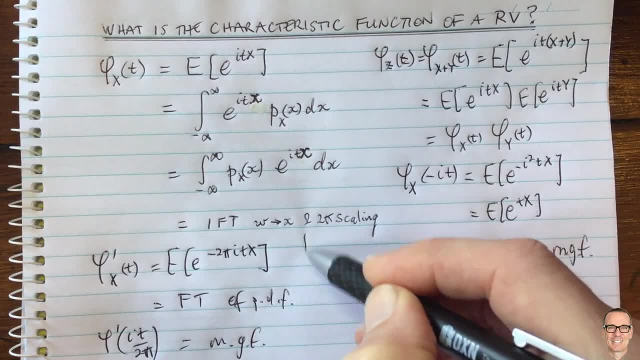 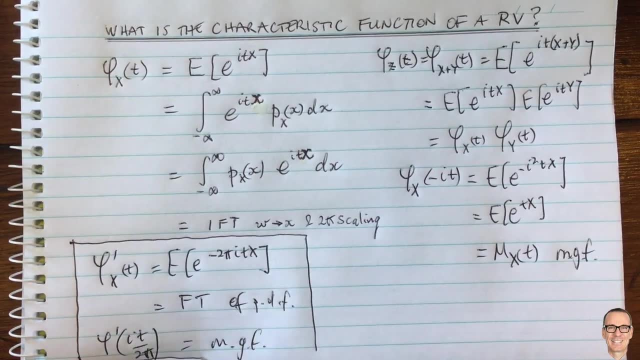 definition here. if we put in i t divided by two pi with this new definition, then we get the moment generating function. So this definition here I'll just put a box around it. This is a different definition, obviously very closely related, just simply with a minus in there. 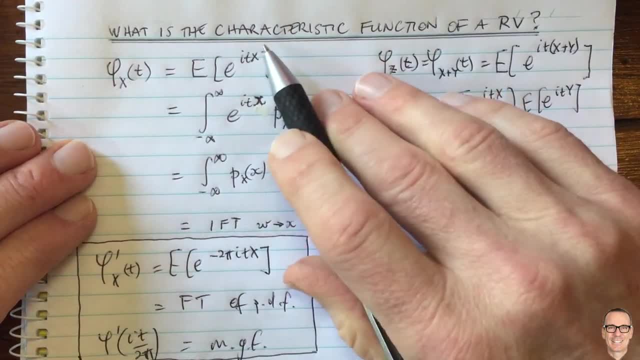 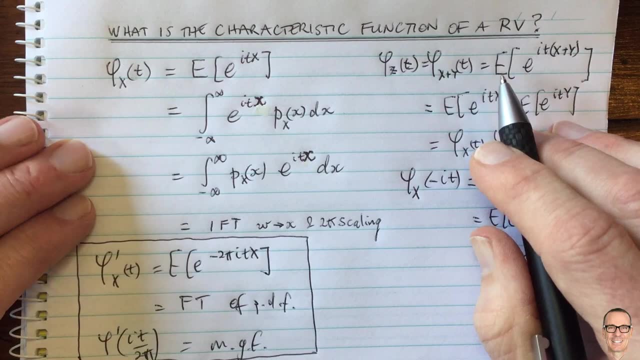 So if this video has helped you to get more insight into the characteristic function and its relationship to the moment generating function and its uses, then give it a thumbs up. It helps others to find the video. Of course, check out the web link in the details below this video. 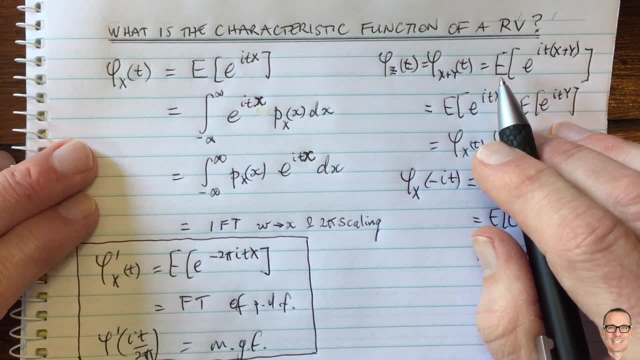 where you'll find a full, categorized list of all the videos on the channel and subscribe to the channel for more videos.